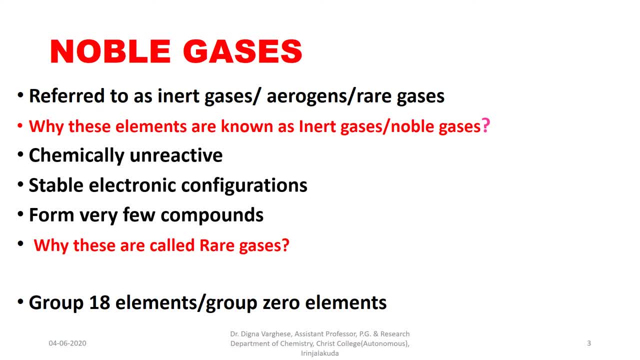 They form very few compounds. Why these elements are known as inert gases or noble gases, Because these are called rare gases. This is because their existence in very minute quantities in the atmosphere. They are also known as group 18 elements or group 0 elements. 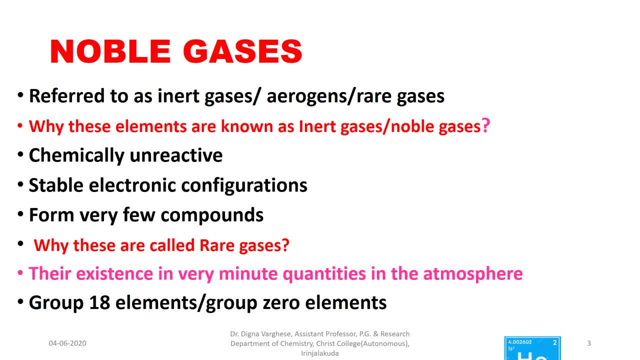 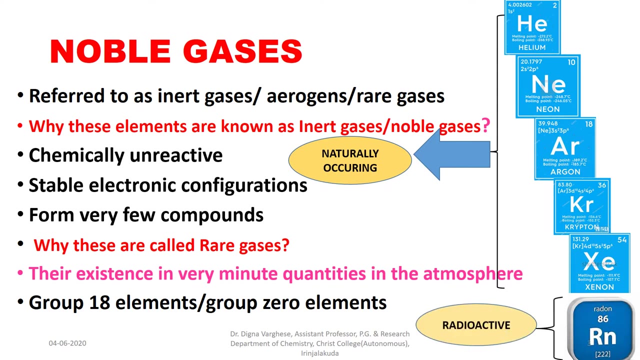 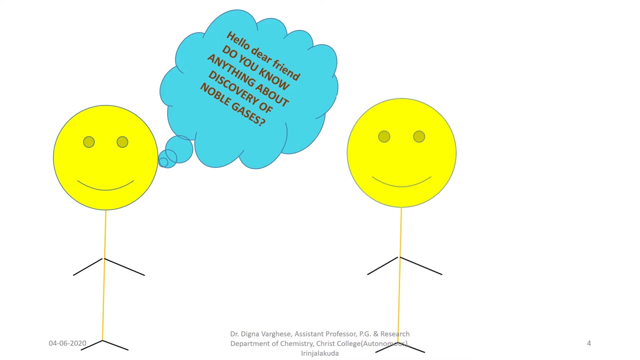 The members of the group. 18 is helium, neon, argon, krypton, xenon. They are naturally occurring When we look at the. They are naturally occurring When we look at the. Do you know anything about discovery of noble gases? 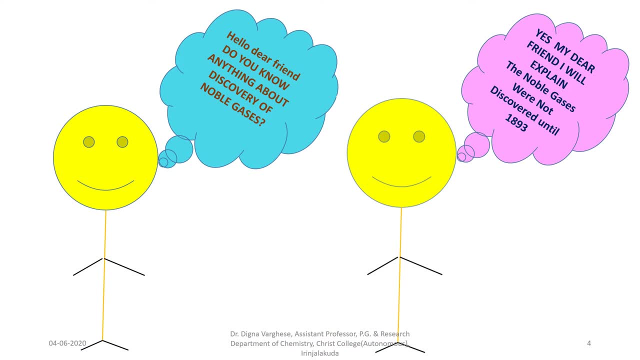 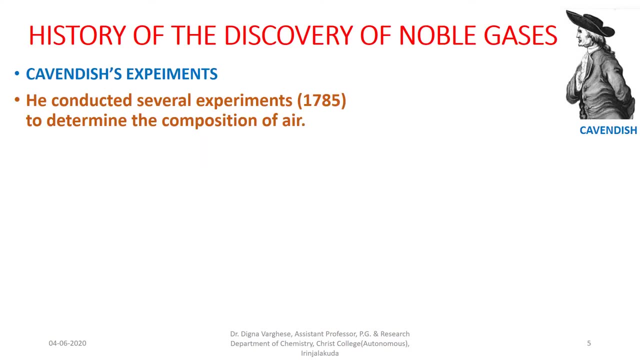 Yes, my dear friend, I will explain. The noble gases were not discovered until 1893. Is it true? history of the discovery of noble gases. first explanation is cavendish's experiments, henry cavendish. he conducted several experiments to determine the composition of air. 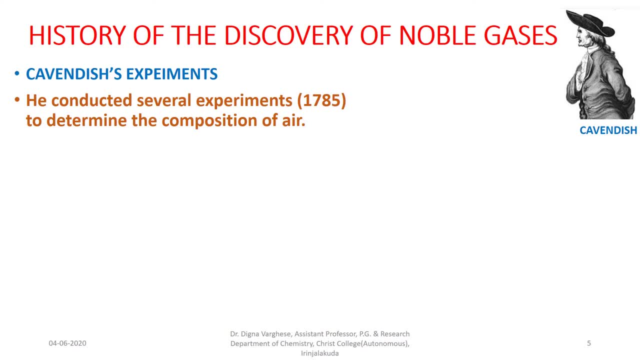 cavendish, who obtained the first experimental evidence for noble gases in 1785. he taken purified air mixed with excess oxygen in a jar and he applied electric spark on it. whole nitrogen converted into nitrogen oxides. the residual gas then passed through first in aqueous potassium hydroxide to absorb carbon dioxide and nitrogen dioxide. 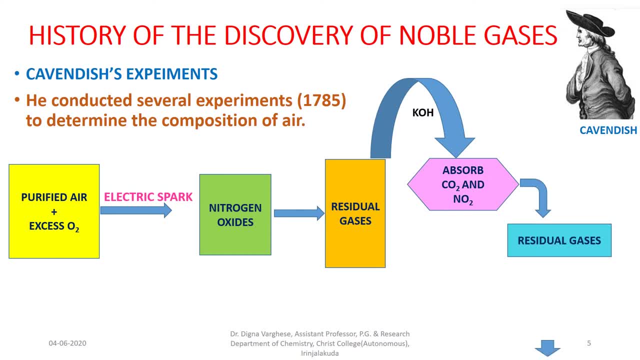 the residual gases then passed into potassium pentasulphide to absorb oxygen, he found that a very small residual part is there. he analyzed this for several years. more than a century later, unreactive fraction was extracted, eventually shown to be a mixture of noble gases. 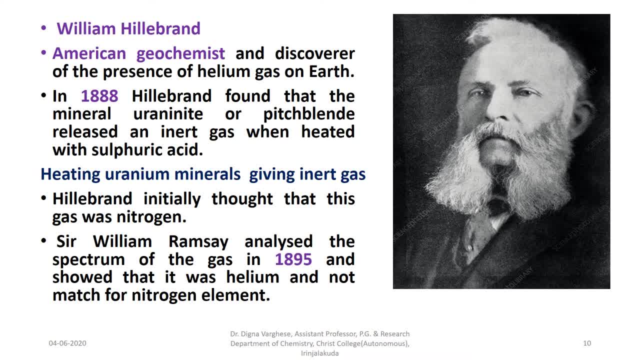 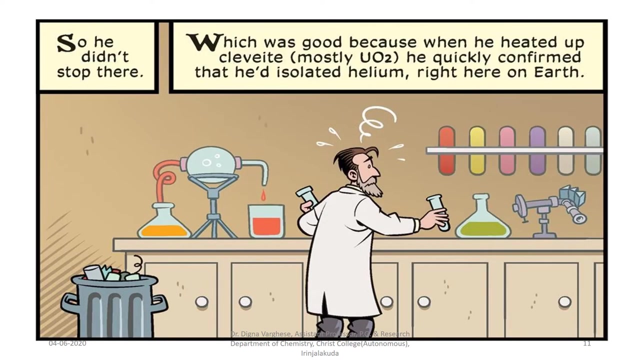 minerals on heating with sulfuric acid, giving inert gas. he thought it was nitrogen, but later Ramsey analyzed this in 1895 and the spectrum showed that it was helium and not much for nitrogen. Ramsey continued his experiments and he heated clevite, that is an uranium. 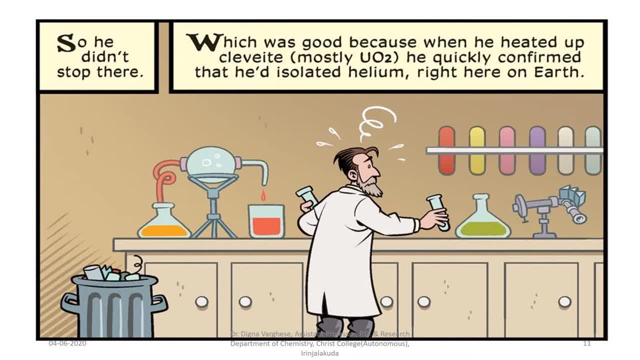 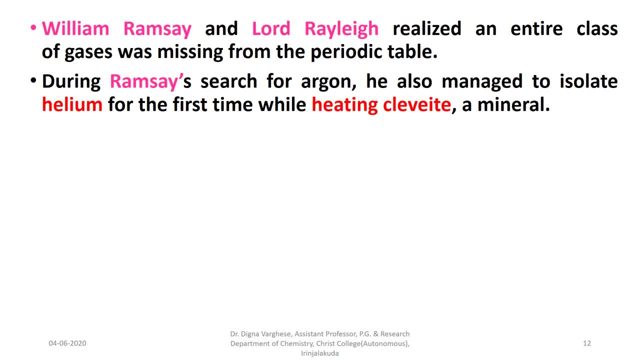 an entire class of gases was missing from the periodic table during Ramsey's from the periodic table during Ramsey's from the periodic table during Ramsey's search for Argon. he also managed to search for Argon. he also managed to search for Argon. he also managed to isolate helium for the first time, while 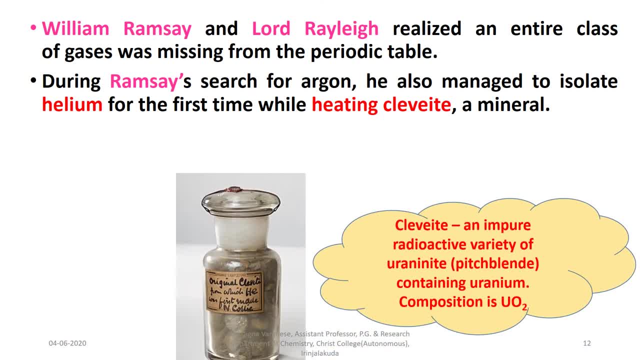 isolate helium for the first time. while isolate helium for the first time while heating clevite in mineral clevite. an heating clevite in mineral clevite. an heating clevite in mineral clevite. an impure radioactive variety of uranium. impure radioactive variety of uranium. 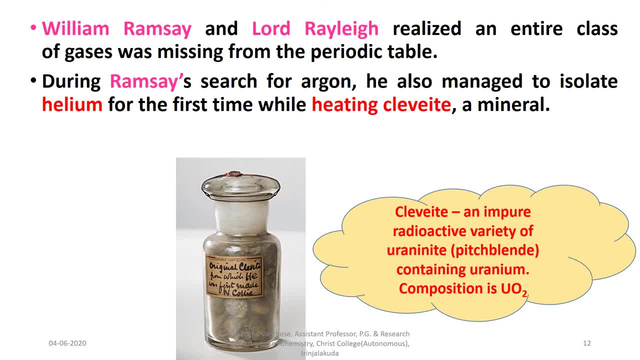 impure radioactive variety of uranium. night containing uranium. the composition: night containing uranium. the composition: night containing uranium. the composition is uranium dioxide in 1888. Hill brand is uranium dioxide in 1888. Hill brand is uranium dioxide in 1888. Hill brand heated clevite. 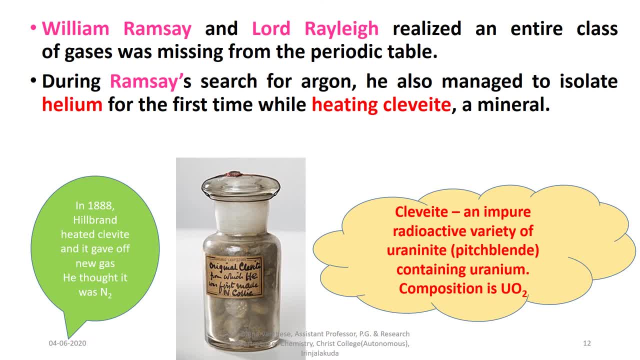 heated clevite and it gave off a new gas at that time. he and it gave off a new gas at that time. he and it gave off a new gas. at that time he assumed that it was nitrogen, but later assumed that it was nitrogen, but later. 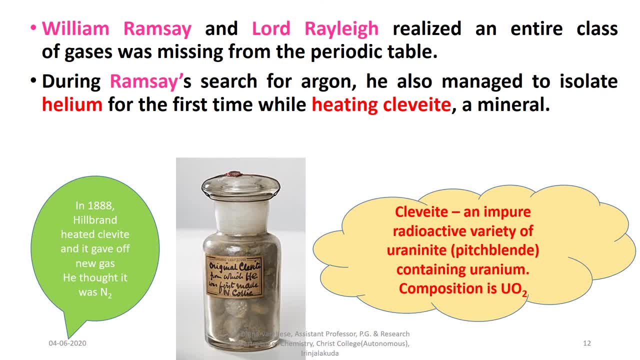 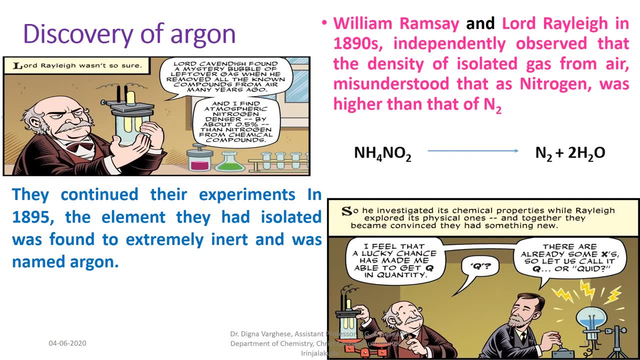 assumed that it was nitrogen, but later Ramsey found that it was helium discovery. Ramsey found that it was helium discovery. Ramsey found that it was helium discovery of Argon. William Ramsey and Lord Rayleigh of Argon. William Ramsey and Lord Rayleigh of Argon. William Ramsey and Lord Rayleigh in 1890s independently observed that the 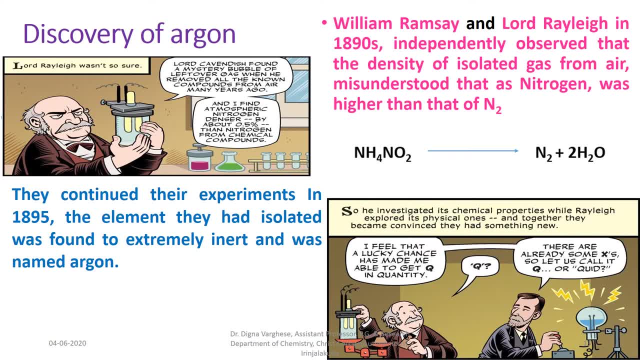 in 1890s independently observed that the in 1890s independently observed that the density of isolated gas from air was. density of isolated gas from air was. density of isolated gas from air was higher than that of nitrogen earlier- higher than that of nitrogen earlier. 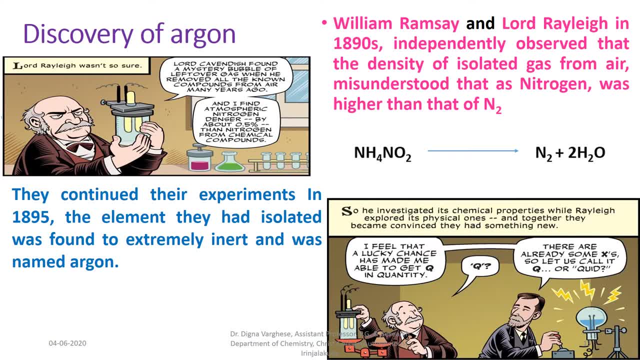 higher than that of nitrogen. earlier experiments showed that some inert gas experiments showed that some inert gas experiments showed that some inert gas is obtained and that was nitrogen but is obtained, and that was nitrogen but is obtained and that was nitrogen, but later Ramsey and Rayleigh explained that. 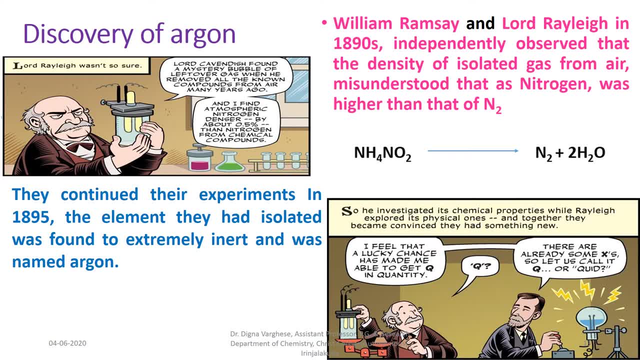 later Ramsey and Rayleigh explained that. later Ramsey and Rayleigh explained that it was not nitrogen because the density it was not nitrogen, because the density it was not nitrogen, because the density of the nitrogen is different from that of the nitrogen, is different from that of the nitrogen is different from that of the inert gas. they continued their 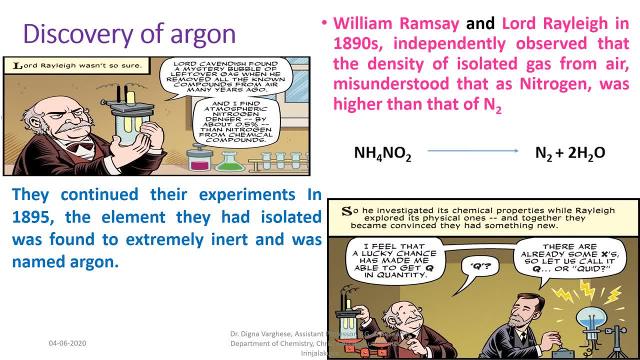 of the inert gas, they continued their. of the inert gas, they continued their experiments in 1895. the element they had experiments in 1895, the element they had experiments in 1895, the element they had isolated, isolated, isolated, was found to extremely inert and was 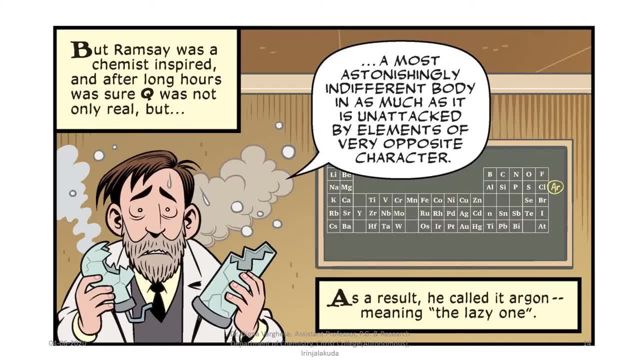 was found to extremely inert and was was found to extremely inert and was named again. Ramsey found that the organ named again Ramsey found that the organ named again Ramsey found that the organ is not attacked by any elements of very is not attacked by any elements of very. 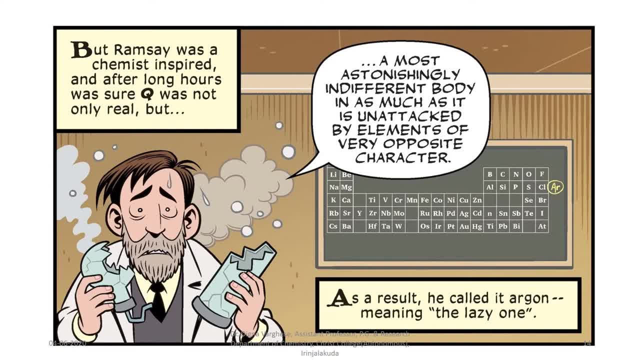 is not attacked by any elements of very opposite character. as a result, he called opposite character. as a result, he called opposite character. as a result, he called it organ. that is from the Greek word it, organ. that is from the Greek word it organ. that is from the Greek word Argos, which meaning lazy one, William. 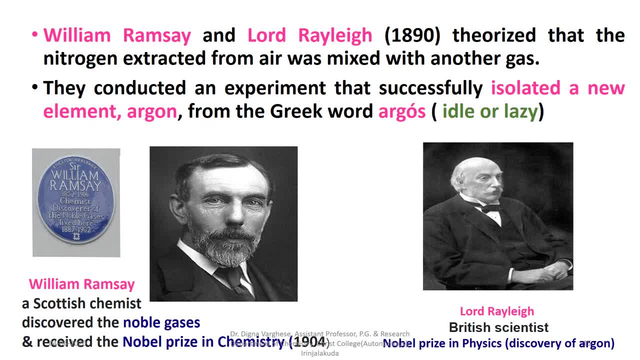 Argos, which meaning lazy one. William William Ramsey and Lord Rayleigh in 1890 theorized that the nitrogen extracted from the air was mixed with another gas. They conducted an experiment that successfully isolated a new element, argon, from the Greek word argos, that means idle or lazy. 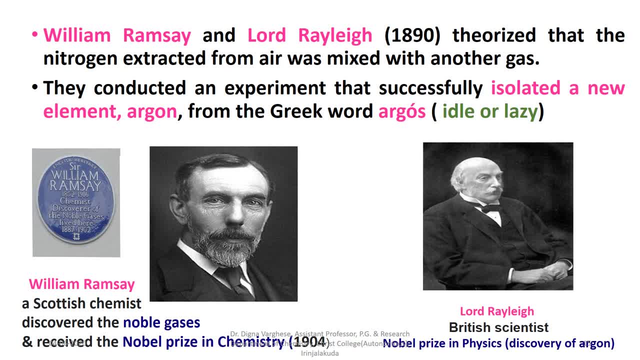 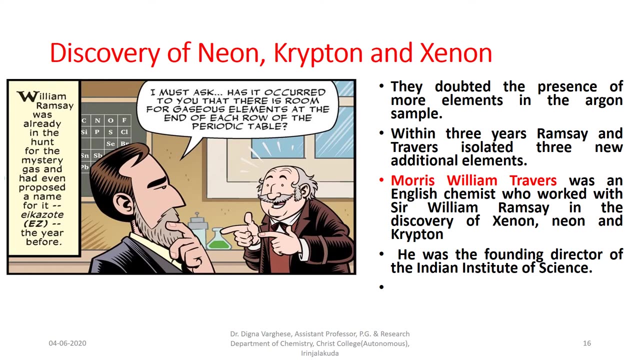 William Ramsey, a Scottish chemist, discovered the noble gases and he received the Nobel Prize in Chemistry. Lord Rayleigh, the British scientist who received the Nobel Prize in Physics, Discovery of Neon, Krypton and Xenon. Rayleigh and Ramsey themselves doubted the 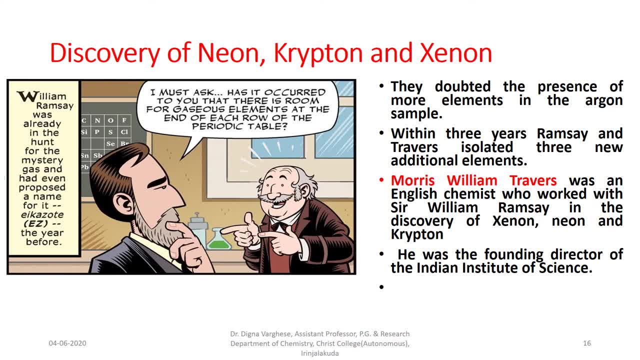 presence of neon, They discovered the presence of more elements in the argon sample itself that they had isolated Within three years. Ramsey and Travers- William Travers. they isolated the three additional elements by low-temperature evaporation of argon obtained by the fractional distillation. 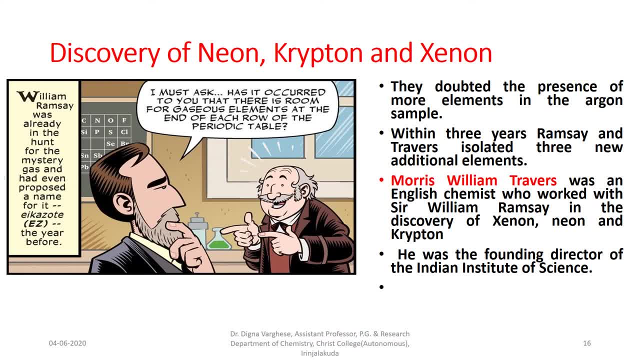 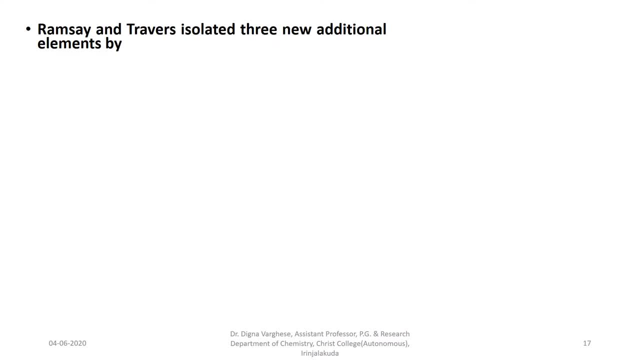 of liquid air. Maurice William Travers was an English chemist who worked with Sir William Ramsey in the discovery of Xenon, Neon and Krypton. Ramsey and Travers isolated three new additional elements by fractional distillation of liquid air, Giving isolation of argon. But then they found that the argon was not isolated. RAMSEY AND TRAVERS WORKED WITH SIR WILLIAM RAMSEY IN THE DISCOVERY OF XENON, NEON AND KRYPTON. RAMSEY AND TRAVERS ISOLATED THREE NEW ADDITIONAL ELEMENTS BY FRACTIONAL DISTILLATION OF LIQUID AIR GIVING. ISOLATION OF ARGON AND ARGON IN THE PARTICULAR STATEMENT. 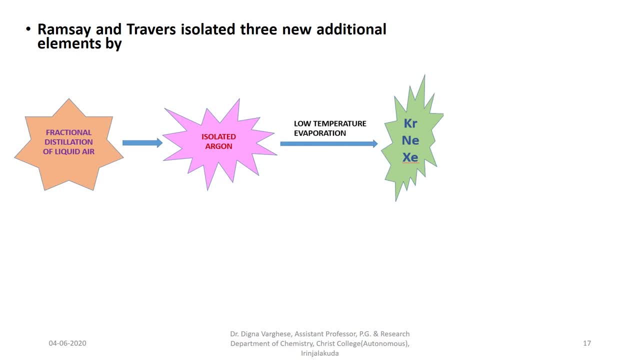 Which, on low temperature evaporation giving a mixture of gases, krypton, neon and xeno, Fractional distillation is the separation of mixture into its components. The chemical components are separated by heating them to temperature at which one or more fractions of the mixture will vaporize. 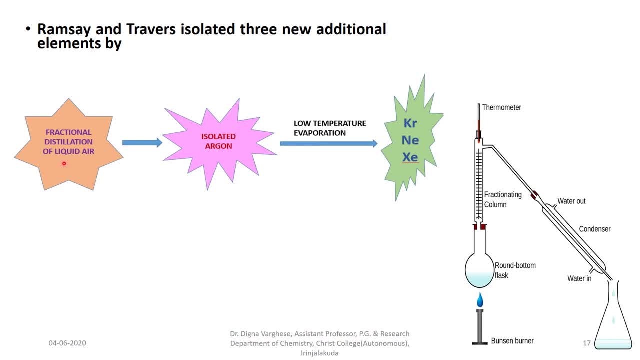 It uses distillation to fractionation. Apparatus required for this fractional distillation is a Bunsen burner which acts as a heat source, a round bottom flask, a condenser- a bix condenser- a fractionating column and a receiving flask. 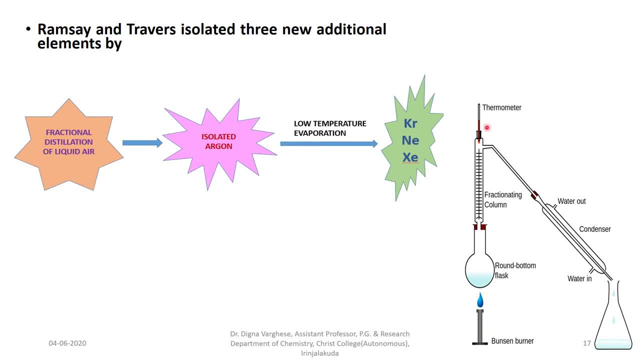 and a thermometer attached to this. This is an ordinary fractional distillation setup. These elements- krypton, neon, xenon- obtained by the low temperature evaporation of the gases. These give independent spectral lines, Those elements named after the Greek words kryptos, for krypton, that means hidden. 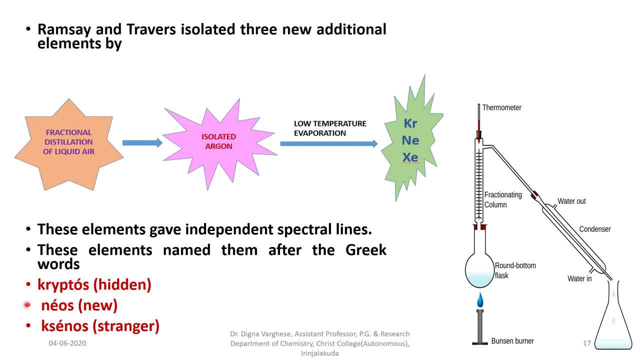 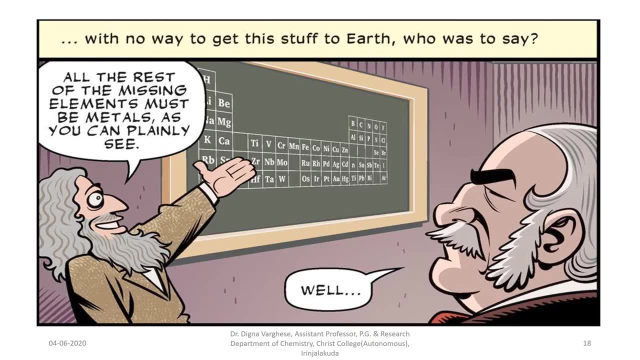 neos for neon, that means new xenos for xenon that means stranger. In the case of earlier periodic table there are some vacant spaces to fill elements, But Mendeleev thought that there are only to find metal. He don't accept anything from Rayleigh. 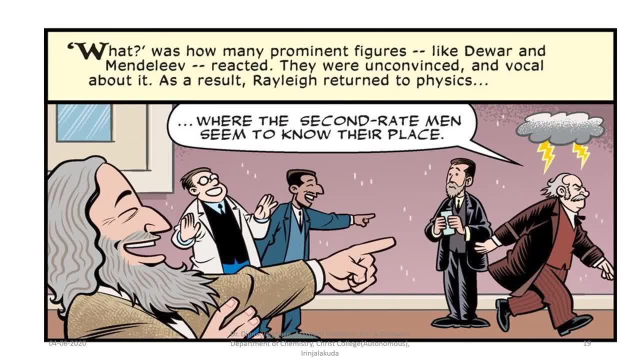 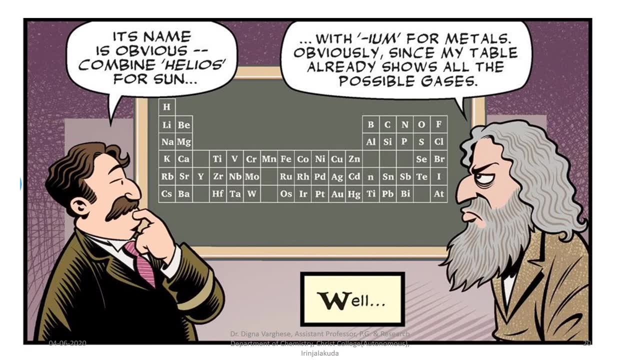 And he and Rayleigh returned to physics. But the scientists who discovered helium and other noble gases, they want to fill separate group in periodic table. But Mendeleev said that IOM for metal only. His thought was his periodic table was already filled by all gases. 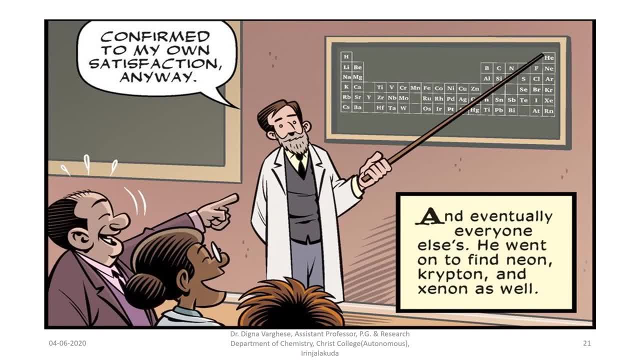 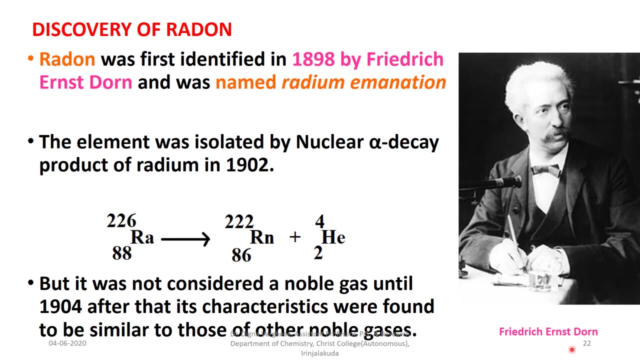 After several confliction and suggestions. later the noble gases were added to the periodic table as zero group elements. Discovery of Radon: Radon was first identified in 1898 by Frederick Ernst Dorn And was named radium emanation. The element was isolated by nuclear alpha decay, product of radium, in 1902. 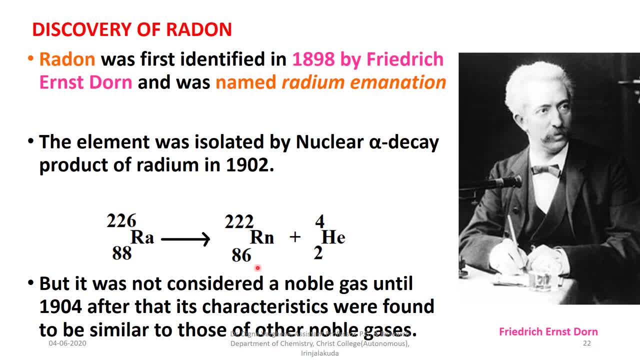 Radium undergoes alpha decay, giving radon and helium. By alpha decay, nuclear charge decreases by 2 units And the mass number of the product decreases by 4 units. But it was not considered as a noble gas until 1904.. After that its characteristics were found to be similar to those of other noble gases. 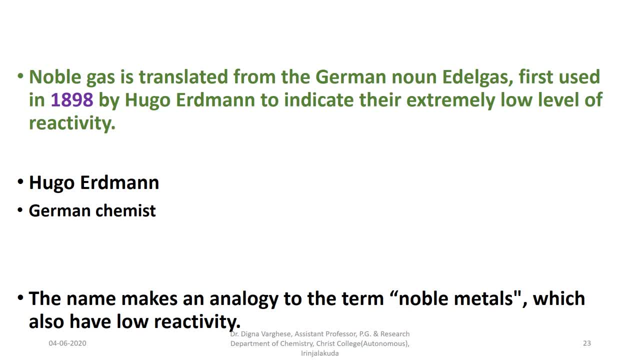 Noble gas is translated from the German noun Edelgas, First used in 1898. By Hugo Edman To indicate their extremely low level of reactivity. Hugo Edman, German chemist, The name makes an analogy to the term noble matters. 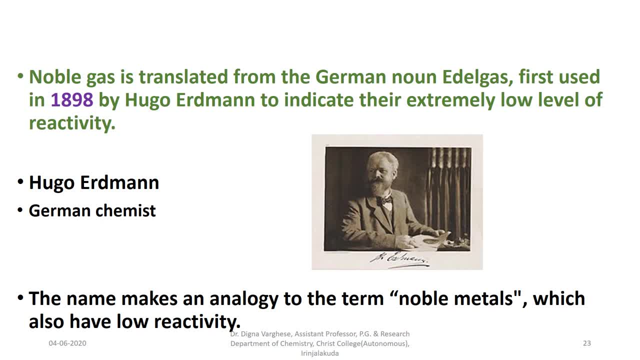 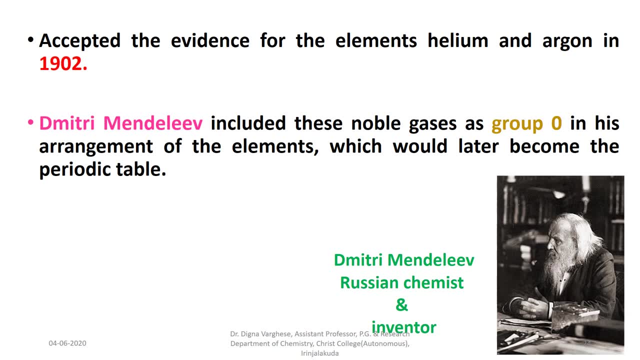 Which also have low reactivity After several years, from 1785 to 1902.. Mendeleev accepted the evidence for the elements helium and argon in 1902.. Dimitri Mendeleev included these noble gases as group zero in his arrangement of the elements. 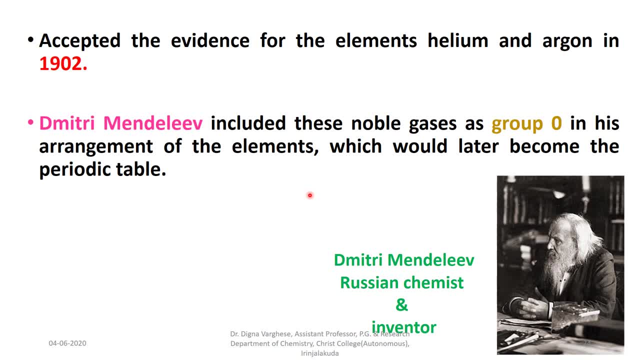 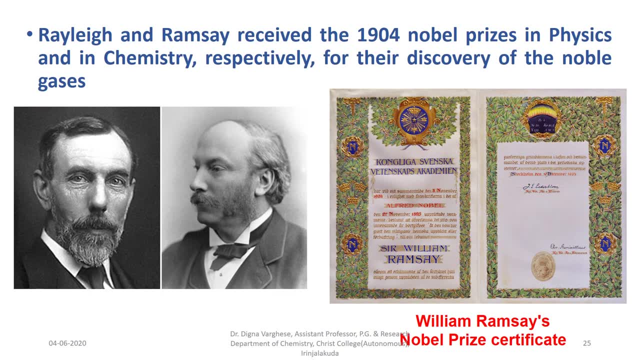 Which would later become the periodic table Dimitri Mendeleev. the Russian chemist and inventor, Rayleigh and Ramsey received in 1904 the Nobel prizes in physics and in chemistry respectively, For their discovery of the noble gas. This is the William Ramsey's Nobel Prize certificate. 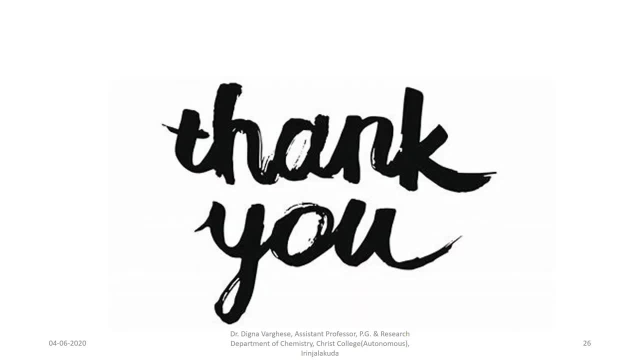 This is all about the discovery of the noble gases. Thank you. 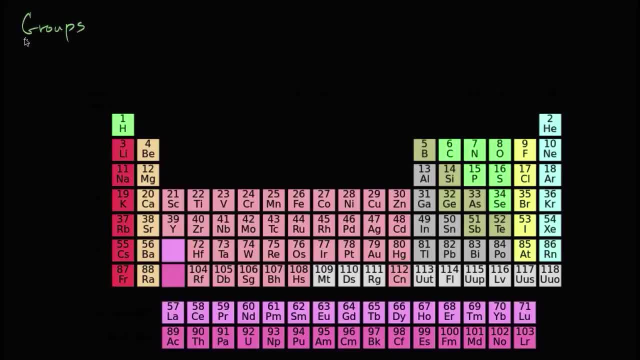 So let's talk a little bit about groups of the periodic table. Now, a very simple way to think about groups is that they just are the columns of the periodic table and a standard convention is to number them. This is the first column, so that's group one. 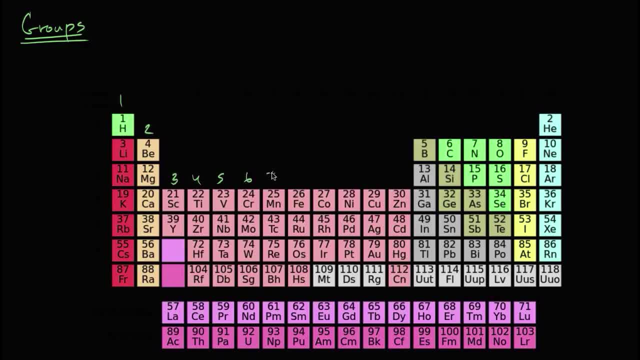 second column, third group, fourth, fifth, sixth, seventh, eighth. group nine: group 10,, 11,, 12,, 13,, 14,, 15,, 16,, 17, and 18.. And I know some of y'all might be thinking: 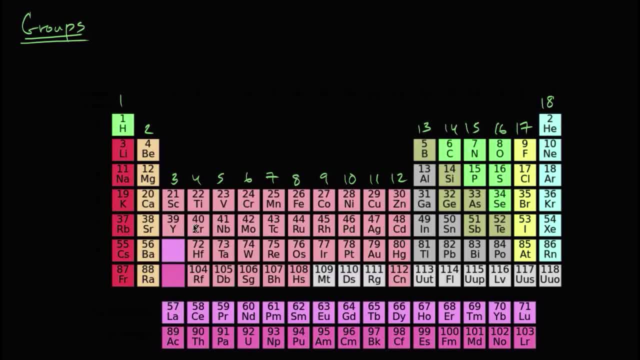 what about these F block elements over here? If we were to properly do the periodic table, we would shift all of these- everything from the D block and P block- rightwards and make room for these F block elements. but the convention is that we don't number them.